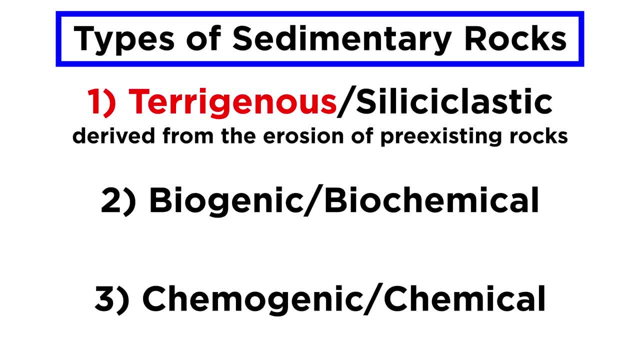 originating from earth. from the Latin terra refers to materials derived from the erosion of preexisting rocks. Siliciclastic refers to materials composed of clasts or fragments of silicate minerals. Pterygianous and siliciclastic are used synonymously, since most pterygianous 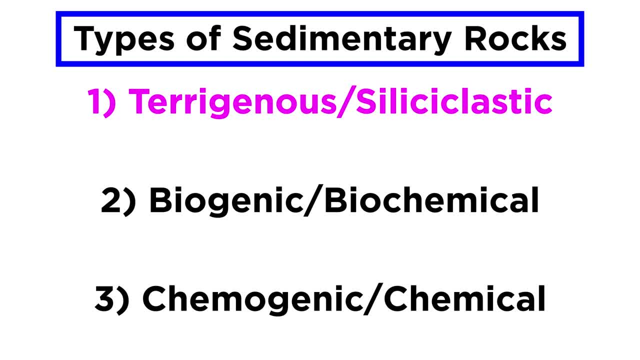 sediments are derived from the erosion of silicate rocks. Biogenic or biochemical rocks are derived from living organisms, both directly and indirectly. Chemogenic or chemical sedimentary rocks are derived from the precipitation of minerals from natural waters, usually involving evaporation in arid climates. 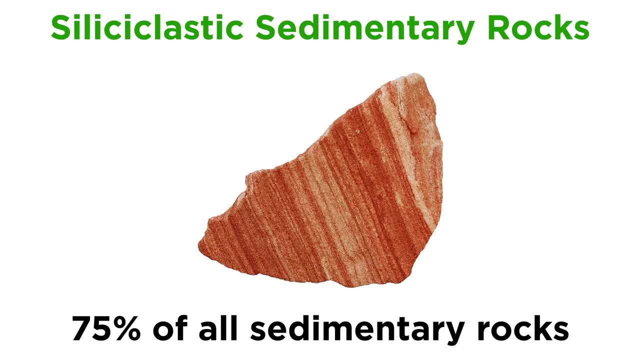 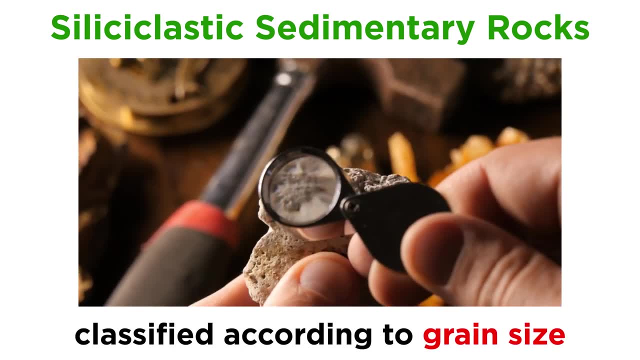 Let's start with the siliciclastic sedimentary rocks, since they are the most abundant, accounting for roughly three-fourths of all sedimentary rocks. In our study of igneous rocks, we learned that one of the first steps in analyzing a hand sample is to determine the grain. 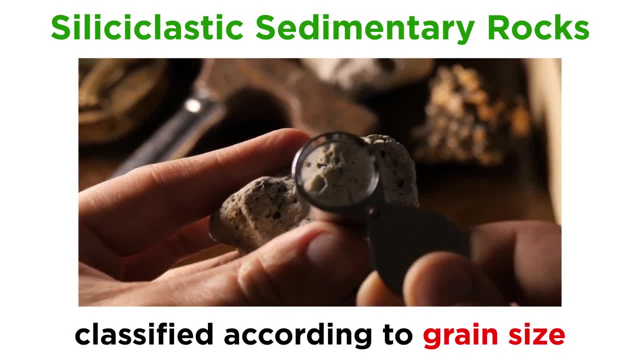 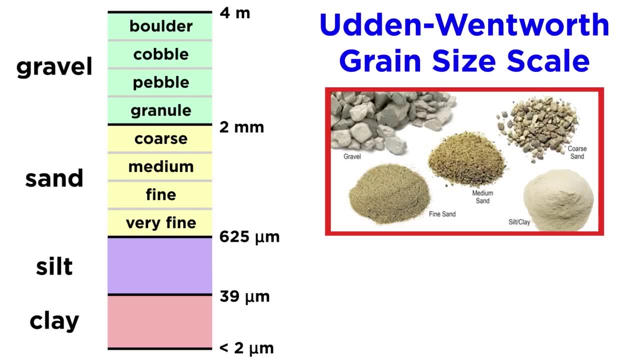 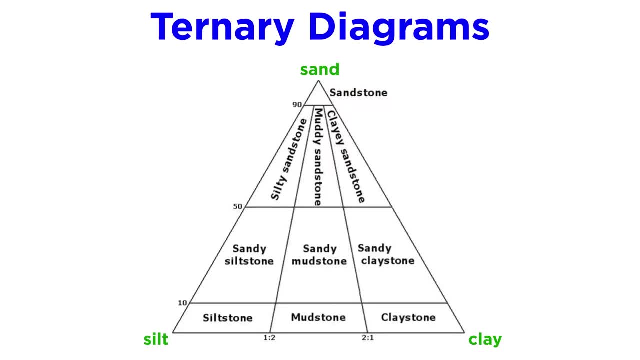 and clay. Geologists often use ternary diagrams to systematically classify rocks. Ternary diagrams represent the relative proportions of three components, in this case different grain sizes. For example, this ternary diagram has the components sand, silt and clay, with 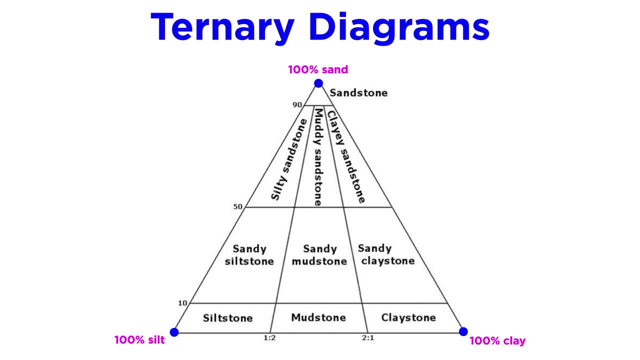 each corner of the triangle, representing 100% of one component. For example, if you were to determine that a sedimentary rock contains 60% sand, 20% silt and 20% clay, it would be classified as a muddy sandstone. It is important to choose the appropriate ternary. 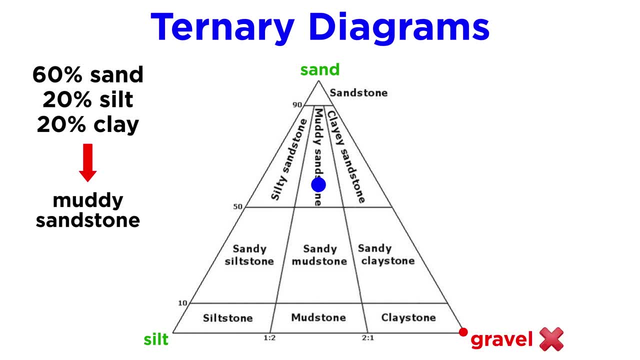 diagram when classifying a rock. For example, you would not use a ternary diagram with gravel as a component for the aforementioned rock, since it does not contain gravel. Furthermore, it is important to recognize that the classification of a rock as a sandstone, silt, silt and 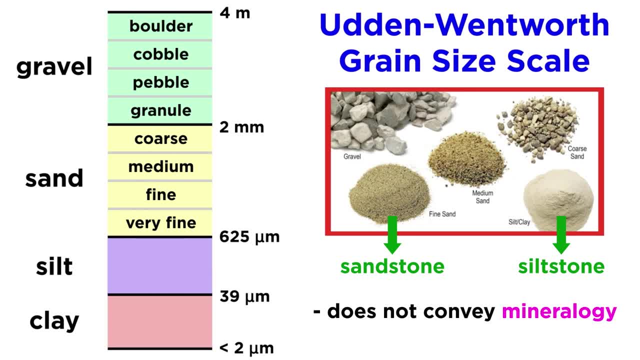 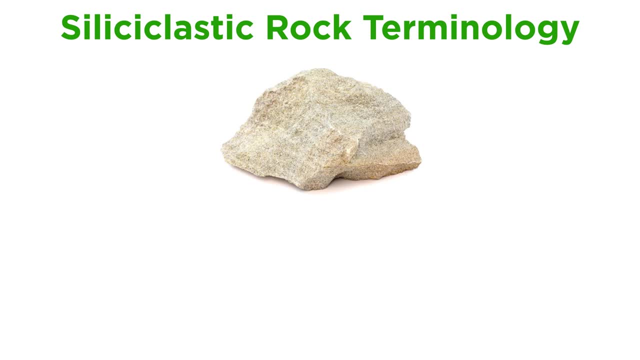 clay, siltstone or otherwise, says nothing about its mineralogy, though it is implied to be siliciclastic, mainly because the biochemical and chemical rocks follow a different classification scheme. Before we explore the main types of siliciclastic rocks, we must cover some terminology, so we 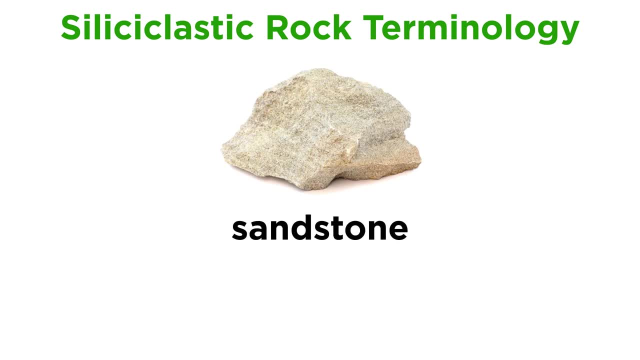 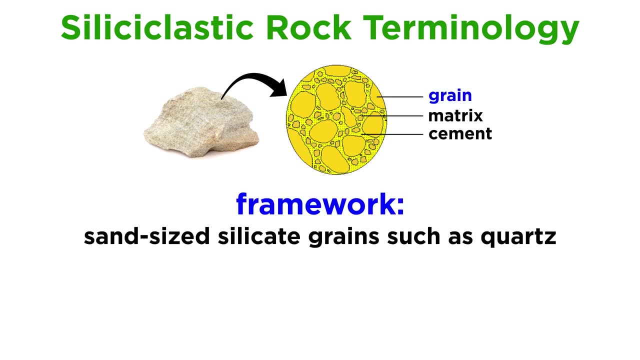 can better describe them. Let's use a typical sandstone as an example. Sandstones consist mainly of sand-sized grains of silicate minerals, often quartz, which make up the framework portion of a rock. Sandstone is a type of rock that is made up of sand, silt, silt and clay. The stones are moved around in a sort of aspical pattern in the shape of a rock. Similarly, the stone wall is made up of a rock and the stones are moved around in a more realistic-looking pattern. The stones are then moved along with the other stones. 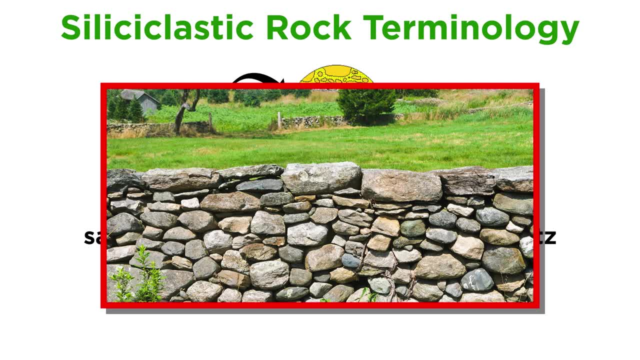 and the stones can be moved together in a more aura-like pattern with a more beautiful formation. This makes them more of a affixable rock. For example, you can see how the rocks are built in a three-dimensional frame. Imagine you are building a stone wall using only the randomly shaped rocks found in a stream. 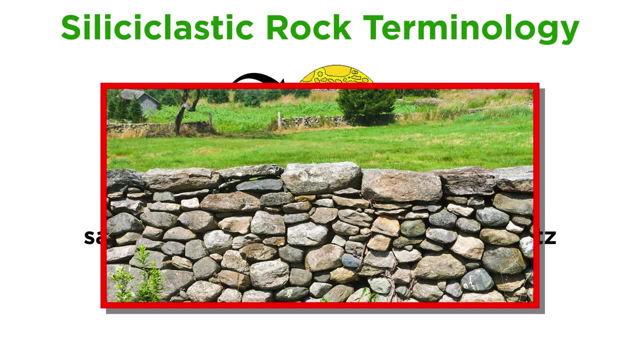 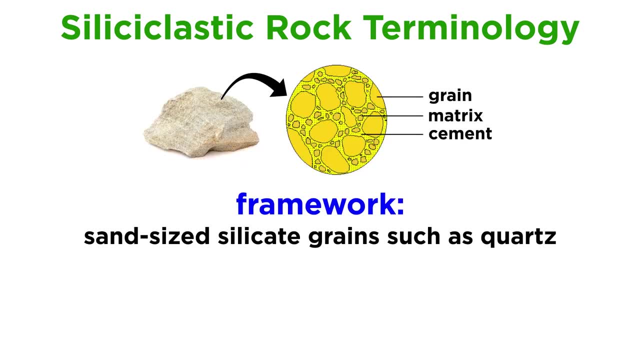 How would they fit together? Obviously, there will be a good amount of empty space between the rocks owing to the fact that random shapes do not perfectly fit together. The same applies to the sand in a sandstone: There is an amount of empty space between the sand grains due 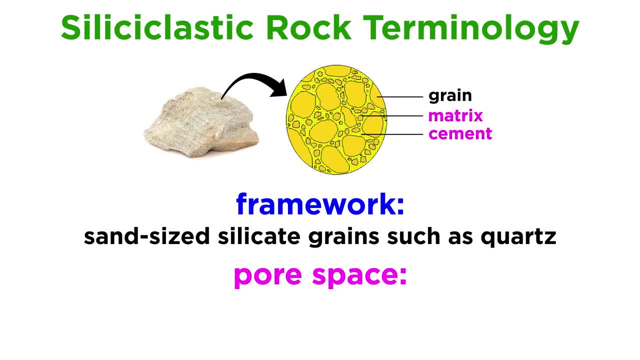 to the way they fit together. This is known as a rock's pore space, and it is often filled with materials to an extent. In some cases, it's filled with fine-grained muds, which is referred to as the matrix portion of a rock. 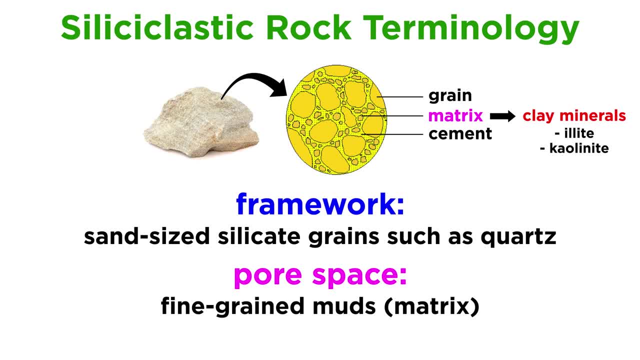 The matrix is commonly composed of clay minerals such as illite and kaolinite. Other times, pores get filled in with minerals that precipitate out of groundwater, called cement. The cement helps glue the rock together, making it harder and more cohesive. 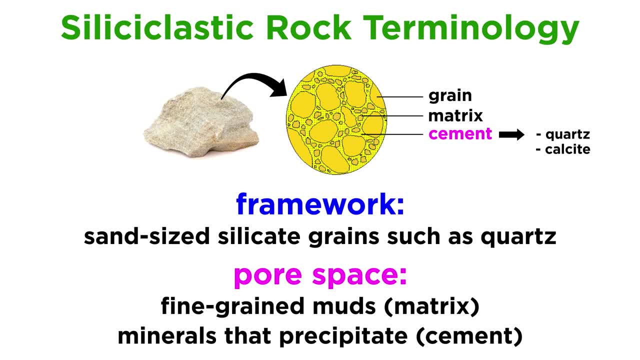 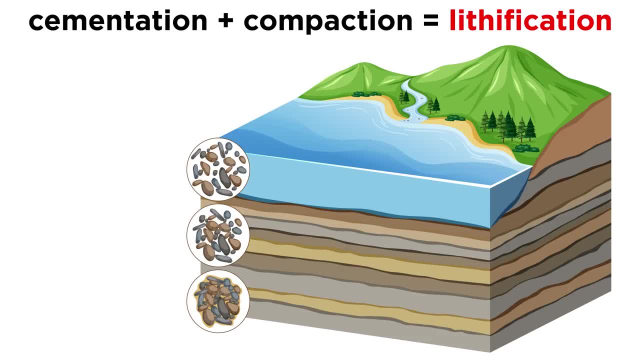 The most common cement-forming minerals are quartz and calcite, with lesser occurrences of the iron oxide minerals and gypsum or anhydrite. Cementation, along with compaction, are together known as lithification, which is the process of converting sediments into sedimentary rock. 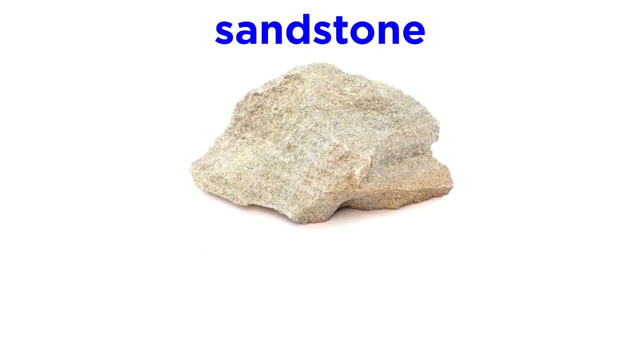 We now have sufficient knowledge to start looking at siliciclastic rocks in more detail. Let's start with sandstone. We already know that sandstone is a rock composed mainly of sand-sized grains, which make up the rock's framework. The most common framework minerals are quartz, followed by feldspar. 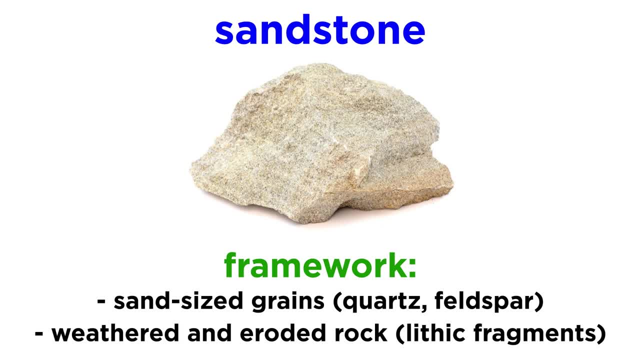 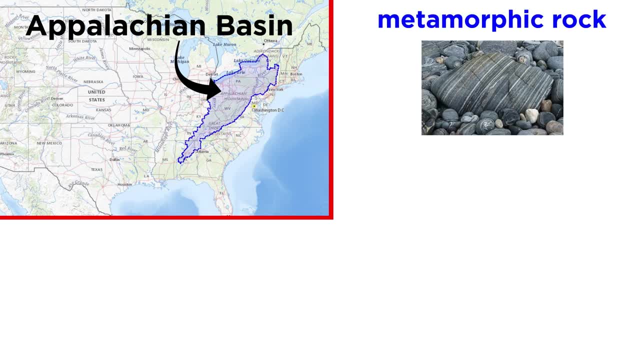 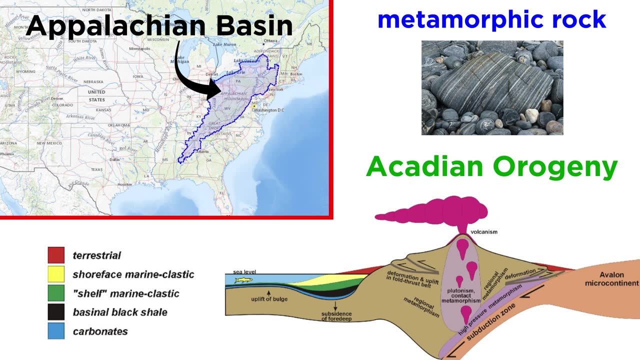 Another common framework constituent are pieces of weathered and eroded rock called lithic fragments. For example, the sedimentary rocks of the Appalachian Basin contain abundant fragments of metamorphic rock derived from the erosion of uplifted metamorphic terrains. Altaplastia, coccidia and all the rest are속alping sandstone. 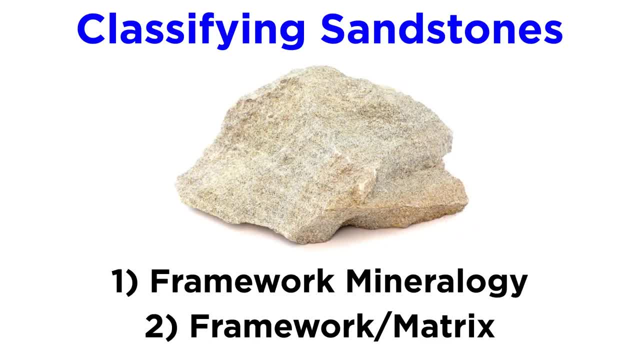 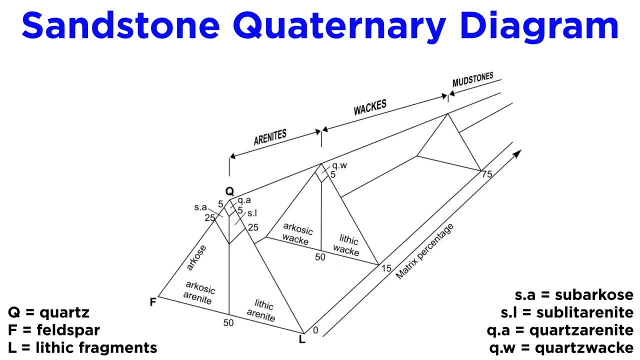 Geologists classify sandstones by combining two properties: framework mineralogy and the proportion of framework to matrix. A quaternary diagram can be used to illustrate the different types of sandstone. Let's start by assuming the amount of matrix is zero. These are known as arenites. 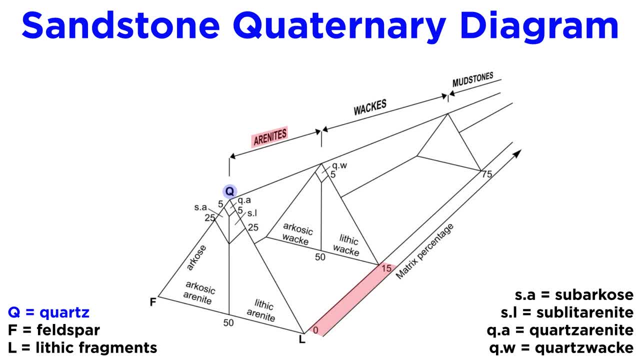 Sandstones that are very rich in quartz are called quartz arenites. If the framework is composed of two types of material, they are called quaternary and cross. the quaternary is the sociedic and the quaternary is the solid. 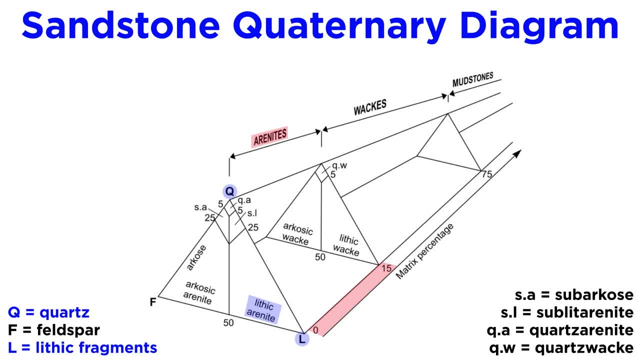 If the framework is composed of two types of material- these are called quaternary and Brookland- mainly of quartz and lithic fragments- it is called a lithic aronite. If it is instead quartz and feldspar, it would be an arcosic or feldspathic aronite. Sandstones with more than 15% matrix are 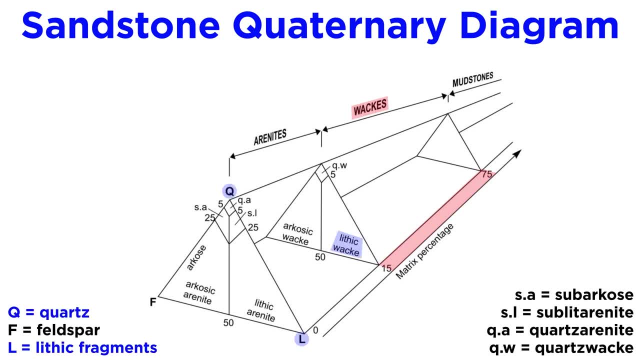 called wackies. so if the framework was dominated by quartz and lithic fragments, it would be classified as a lithic wacky and so forth. Sedimentary rocks with more than 50% matrix are considered mudstones. Recall from the previous tutorial that feldspar is unstable. 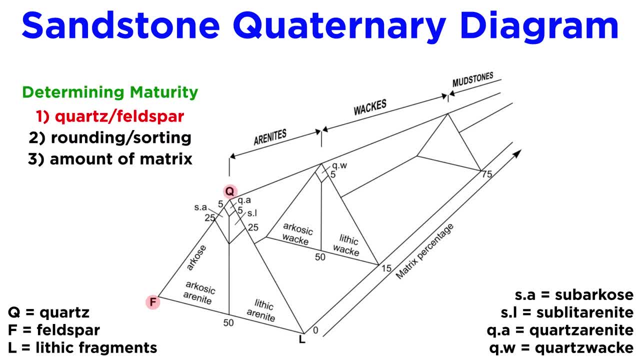 in weathering environments and alters to clay over time. The relative concentration of stable materials, such as quartz, to unstable materials, such as feldspar, is used in conjunction with the degree of rounding, sorting and amount of matrix to determine a sandstone's maturity. 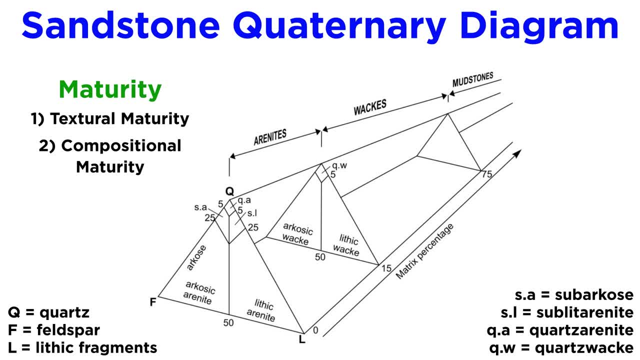 More specifically, maturity is broken down into two categories: textural and compositional. and compositional: Compositionally mature sandstones are depleted in materials that are thermodynamically unstable in weathering environments, including most igneous and metamorphic minerals, except for quartz. Consequently, they tend to be quartz aronites. 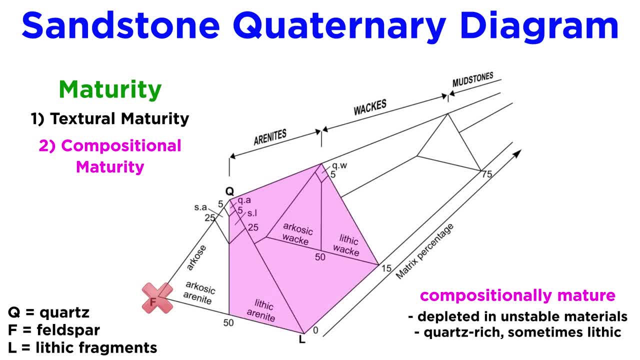 and quartz wackies, though they can occasionally be lithic aronites or lithic wackies if the lithic fragments are quartz-rich, such as chert or quartzite. Compositional maturity indicates that a rock is a quartz-rich rock and that a rock is a quartz-rich rock. 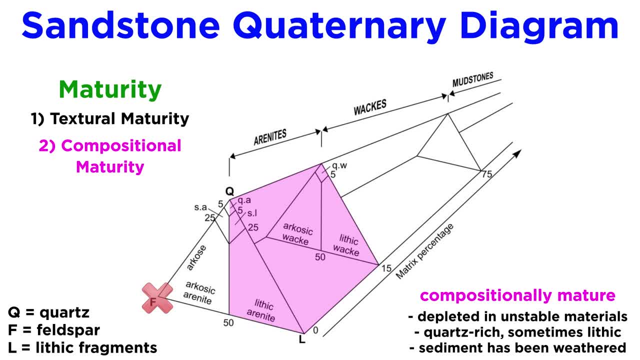 Sediment has spent a great deal of time in a weathering environment, prior to deposition and burial, sufficient to chemically alter unstable sediments. We will talk more about chemical weathering in a later tutorial. Texturally mature sandstones have well-rounded and well-sorted grains. 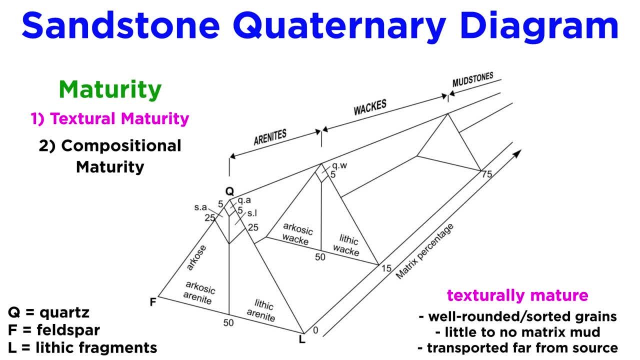 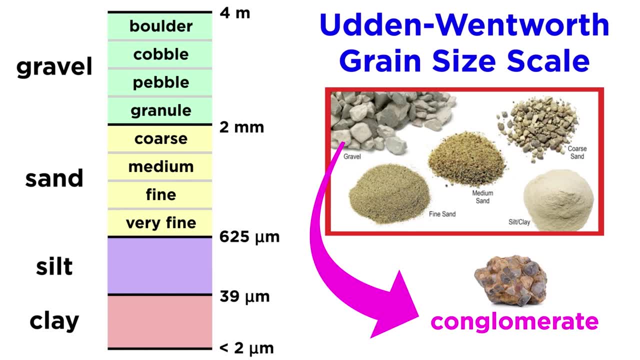 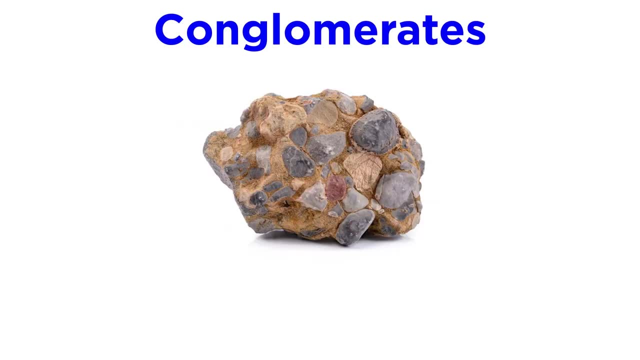 with little to no matrix mud, indicating great transport distance from source to burial. Let's move on to the coarsest-grained sedimentary rocks conglomerates. Conglomerates are composed of at least 30% gravel-sized particles. True conglomerates. 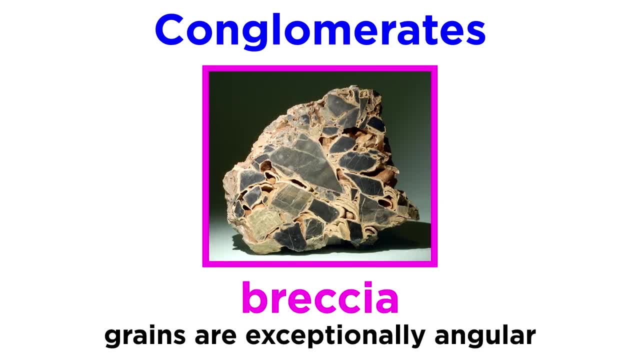 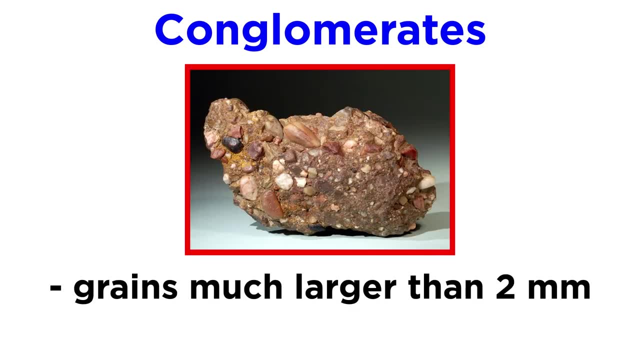 have well-to-subrounded clasts, whereas the term breccia describes a conglomeratic rock that is composed of angular clasts, Since it is relatively uncommon for rocks to contain mineral grains larger than 2 mm, most conglomerate gravels are composed of lithic fragments rather. 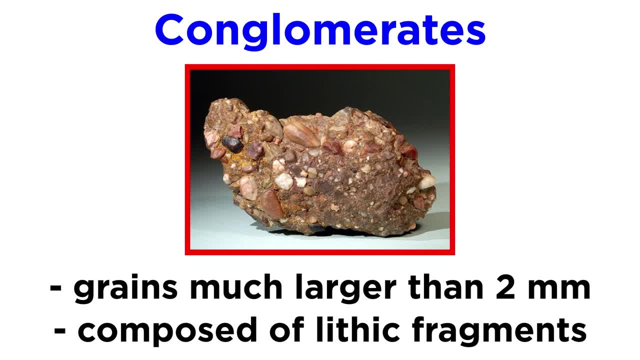 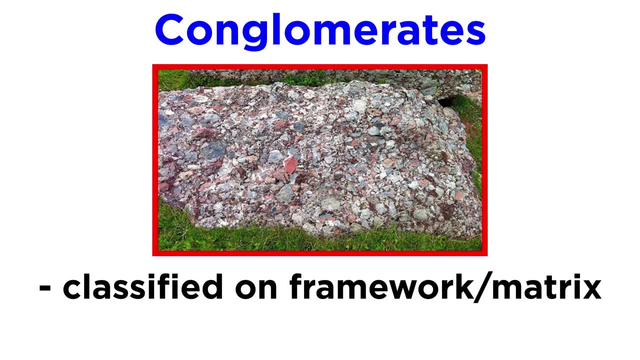 than monocrystalline grains, as is typically the case for quartz. Conglomerates are classified based on the proportion of framework to matrix, similar to sandstones. True conglomerates contain very little matrix and are framework-supported, meaning that gravel-sized clasts are touching When a conglomerate is matrix-supported. 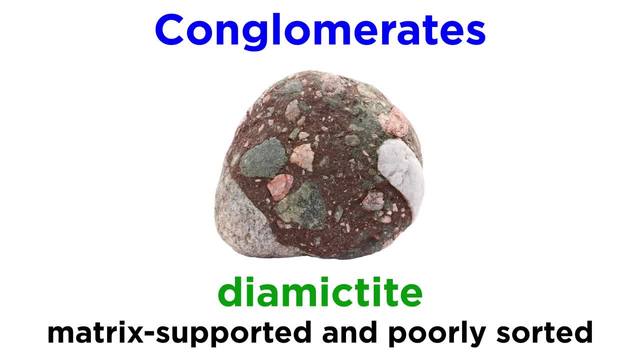 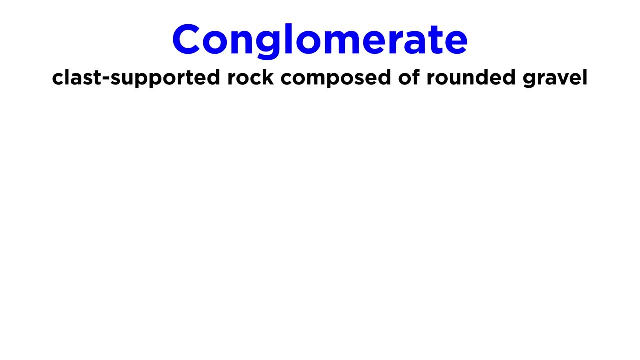 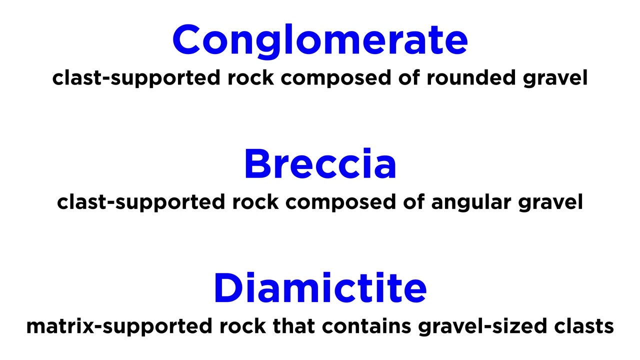 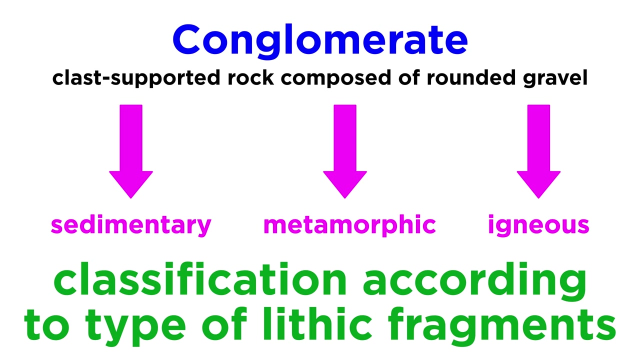 it is called a diamictite, with diamictite meaning mixed rock. Diamictite is a general term for extremely poorly sorted geologic material in a muddy matrix. Diamictite means flat and silty rock, and it means both flat and silty When it is. 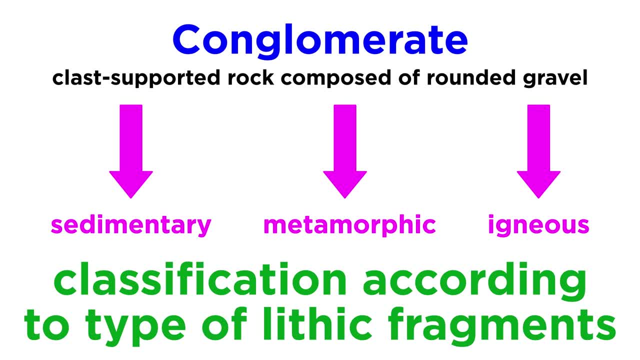 modified, it is called a conglomerate. Mantrix can also be classified as a conglomerate. The conglomerate can be classified as a conglomerate because it is compact and is the same size as a rock. the type of lithic fragments that comprise the framework fraction mainly distinguishing. 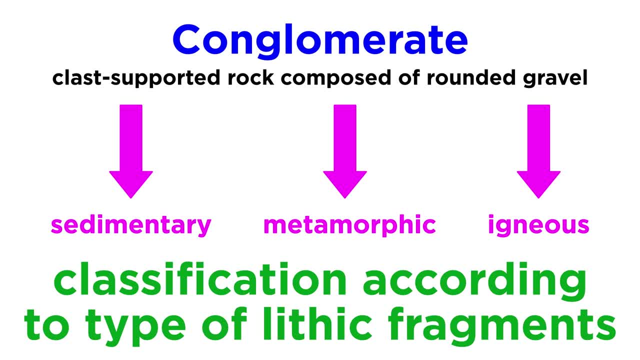 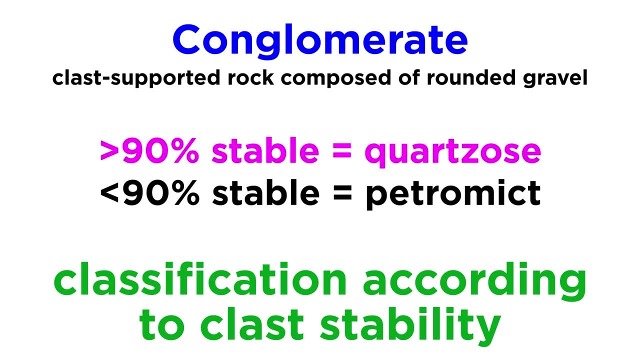 sedimentary, metamorphic and igneous clasts. Additionally, they can be classified based on clast stability, similar to sandstone maturity. Conglomerates with greater than 90% stable clasts are said to be quartzose, while those with less than 90% stable clasts are said to be petromyct. 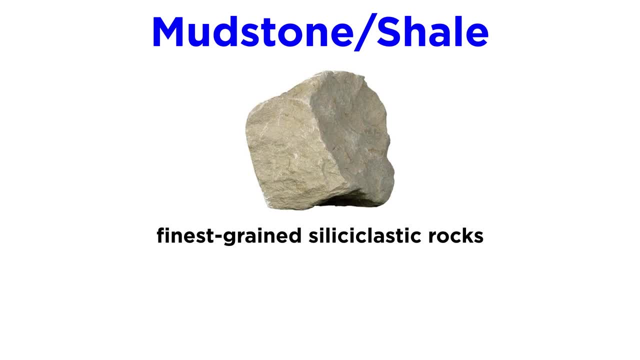 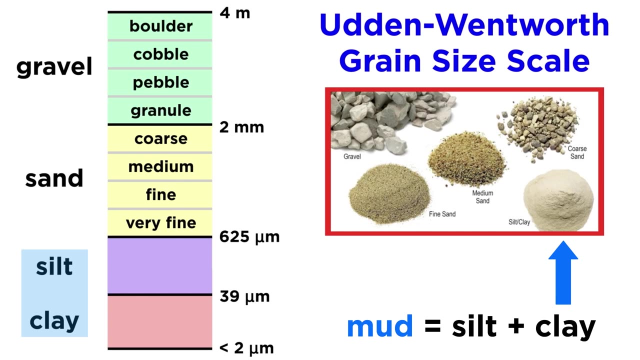 Last but not least are the mudstones and shales, which are the finest grained variety of siliciclastic rocks. More than half of all sedimentary rocks are mudstones, compared to about 20% for sandstones and only 1% for conglomerates. Recall that mud is a general 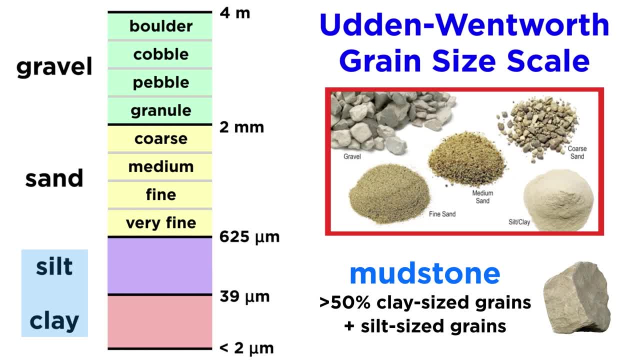 term for silt and clay-sized grains. Hence, mudstones are composed of more than 50% clay-sized grains, with silt-sized grains making up most of the rest. Conglomerates with their very coarse grains are deposited in the highest energy. 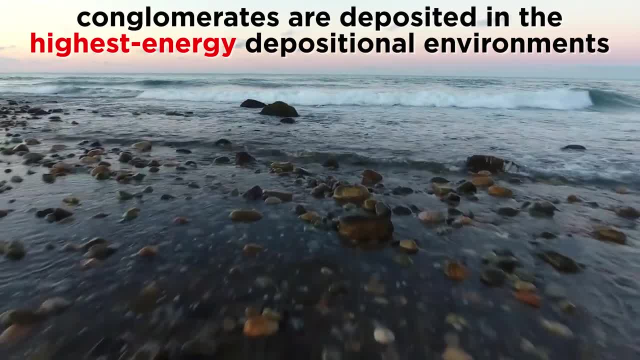 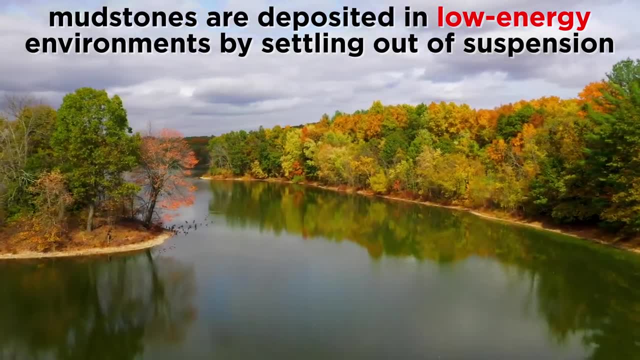 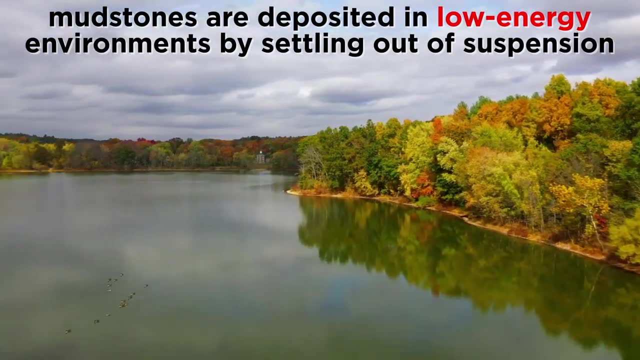 depositional environments like rocky beaches and braided streams. At the other end of the spectrum are mudstones, which can only be deposited in low-energy environments where fine-grained sediments are able to settle out of suspension. The largest mudstone deposits form in the deep 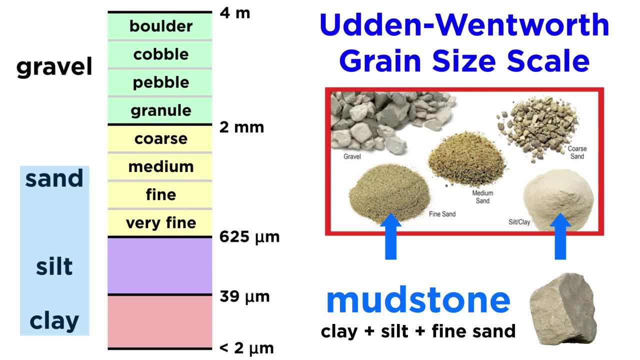 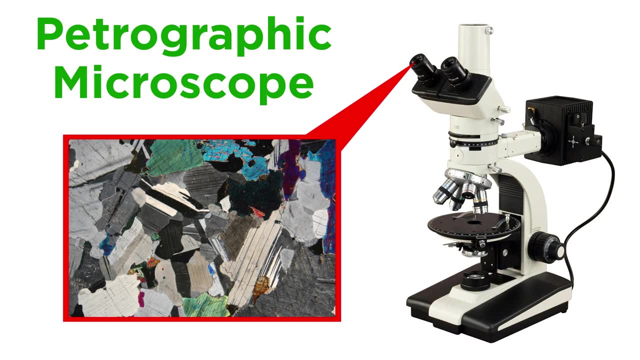 calm waters of lakes and oceans. It is not uncommon for clay, silt and fine sand rocks or salt to be simultaneously present in a mudstone, elevating the importance of proper grain size classification. This can be done accurately with a petrographic microscope. 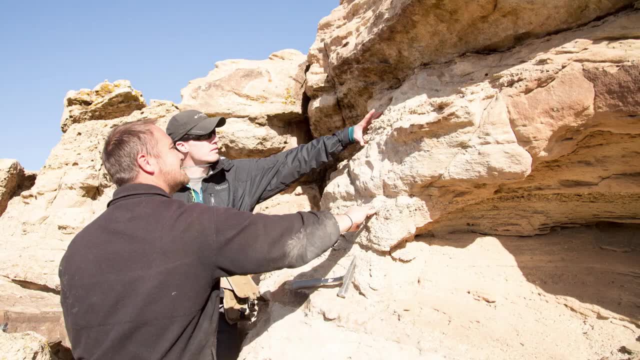 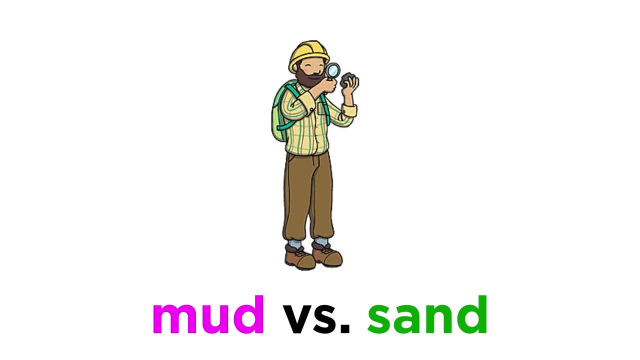 though the clay-sized grains will be too small to resolve. Field geologists have a few tricks for determining grain size. Mud can be easily distinguished from sand based on whether grains are visible to the naked eye, since anything smaller than fine sand is too small to be seen. 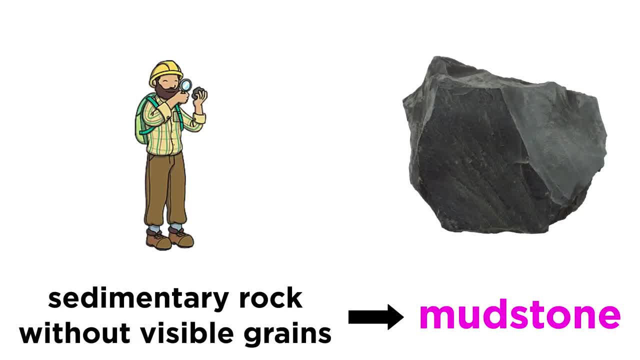 So, in order to reports, mud should have a selected ground that is 2.25 feet wide. So if we have a sedimentary rock or much more, 57.9 feet will be a good. So if we have a sedimentary rock without visible grains, it would be classified as. 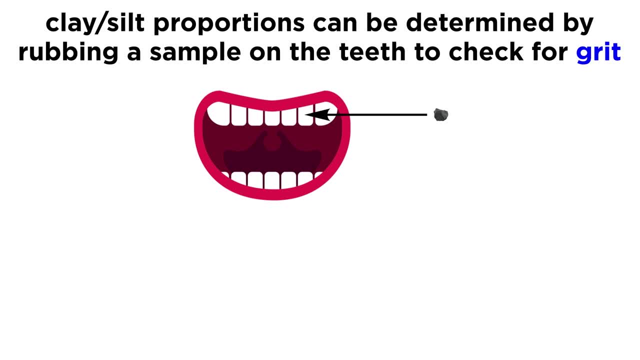 a mudstone. Furthermore, the relative proportions of clay to silt can be determined by rubbing a small sample over your teeth to determine the amount of grit present. If little to no grit is detected, it is probably nearly pure clay and would be classified in. 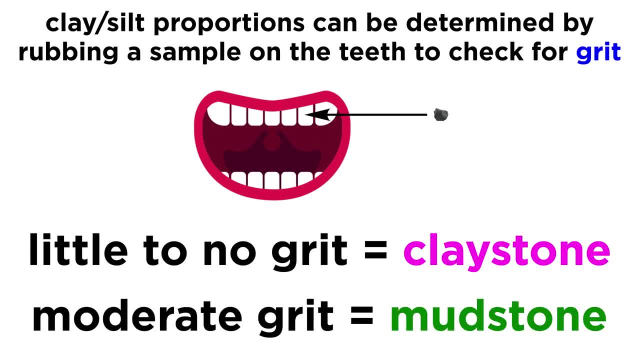 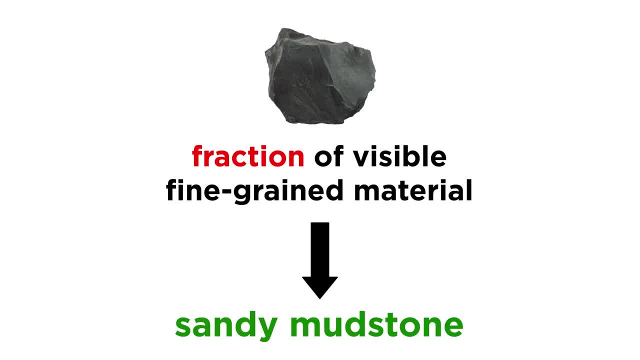 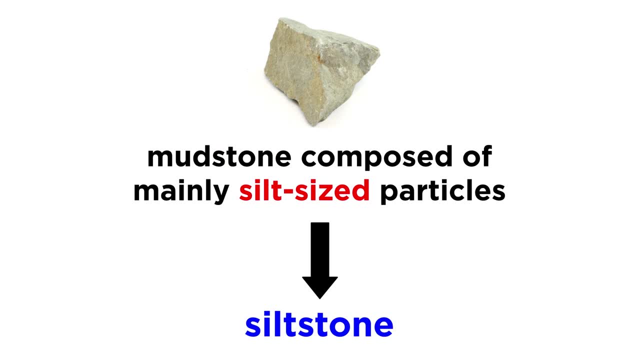 the field as a claystone. If moderate grit is present, that will suffice to classify it as a general mudstone. If a mudstone contains a fraction of visible fine-grained material, it would be classified as sandy mudstone. Siltstone is a more specific type of mudstone, being mainly composed of silt-sized particles. 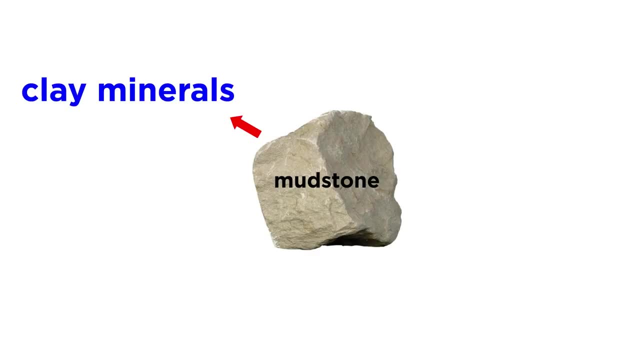 Compositionally, mudstones are primarily composed of clay minerals, with moderate amounts of silt-sized quartz and feldspar. There are several types of clay minerals, including illite, chlorite and kaolinite. They are a product of the chemical composition of the clay and they are a product of the 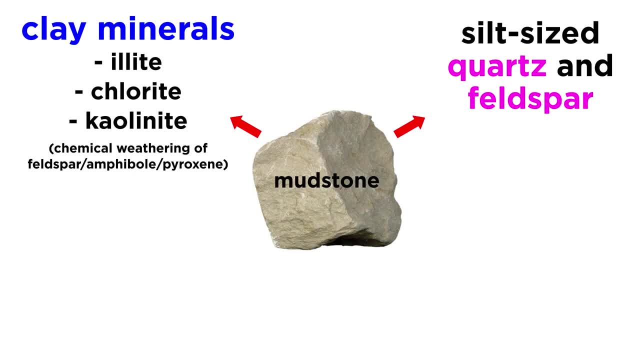 chemical composition of the clay. weathering of primary silicate minerals such as feldspar, amphibole and pyroxene Mudstones can be quite complex mineralogically, containing minor amounts of several other minerals, especially the carbonate, sulfide and oxide-slash-hydroxide groups. They can 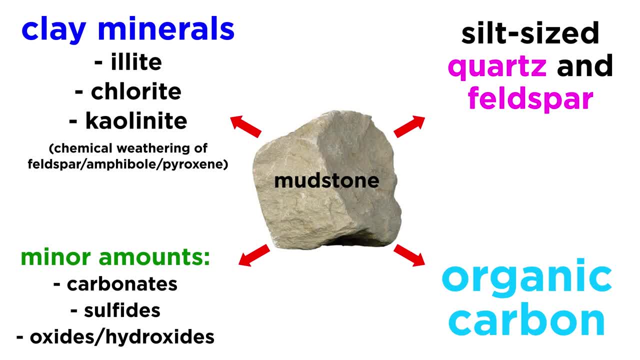 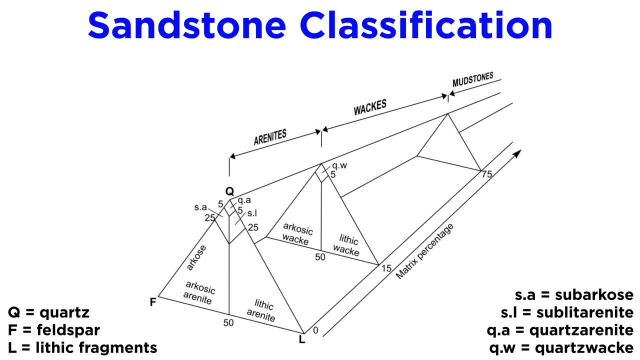 also be quite rich in organic carbon, making up an enormous fraction of global source rocks for oil and gas extraction. The classification of mudstones isn't as straightforward as that of sandstones, which can be easily classified by plotting compositional and textural properties. 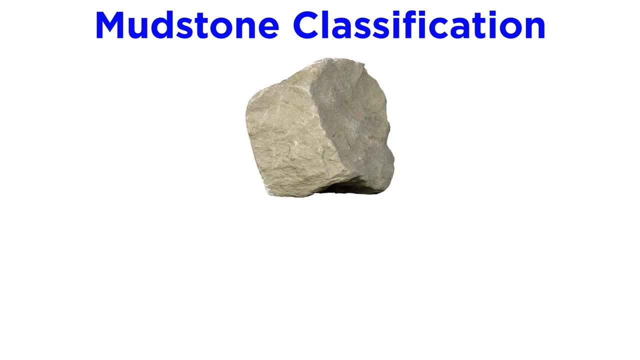 on ternary diagrams. Classifying mudstones involves stringing together descriptive terms. For example, a mudstone that is rich in organic carbon with abundant fossils would be classified as a fossiliferous, carbonaceous mudstone. Mudstones rich in organic carbon tend to 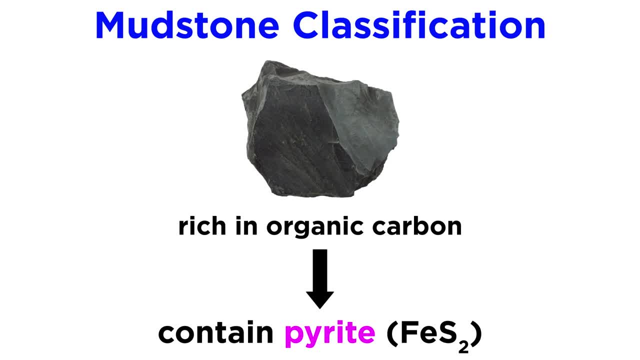 be black in color and often contain pyrite or FeS2.. If a mudstone is fissile, meaning it easily breaks into planar sheets, it is called a shale- the term most non-geologists probably know, rather than mudstone. If a mudstone contains 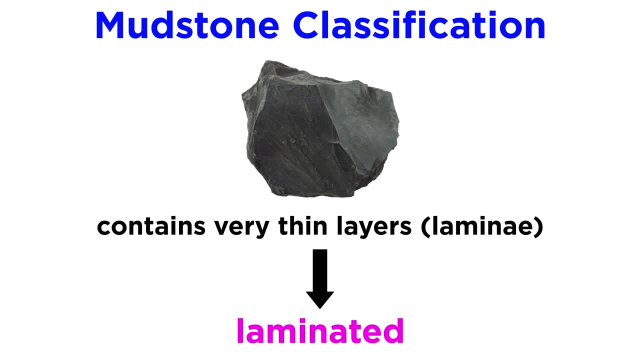 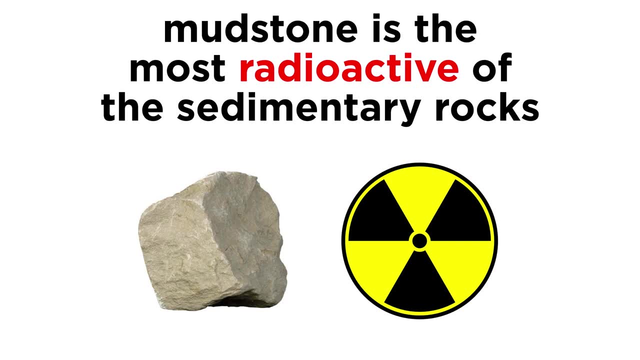 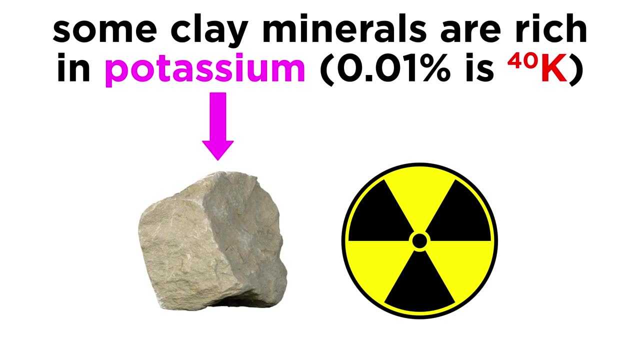 very thin layers called laminae. it is said to be laminated. Another interesting property of mudstone is that it's the most radioactive of the sedimentary rocks. There are a few reasons for this. First, some clay minerals are rich in potassium and 0.01% of potassium.